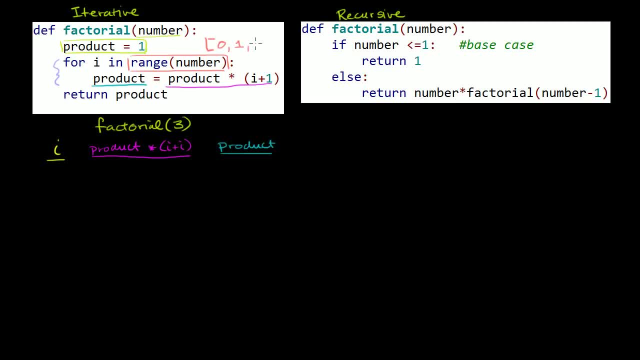 it will literally return a list: 0,, 1,, 2.. So 3 elements starting at 0.. The last element is 3 minus 1.. It is 2.. And so each loop through this for loop i is going to be assigned to each successive element. 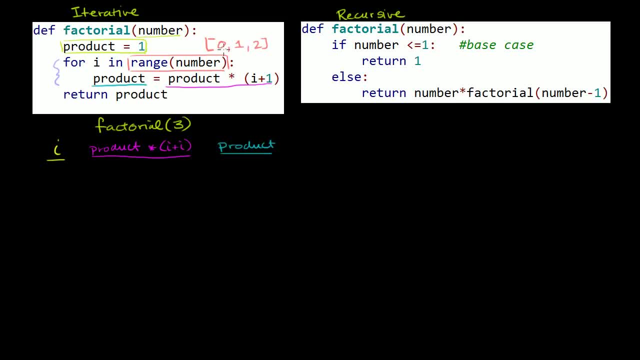 in this list. So on the first time through this for loop, i is going to be assigned to 0. So our i is going to refer to 0. And then product times: i plus 1.. Well, in this first loop, product up here: 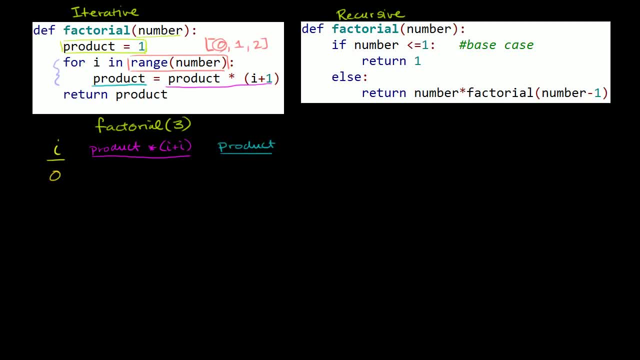 before we even entered the loop, product was defined to be 1.. So product is going to be 1.. And it's 1 times 1 times i, which is 0, plus 1.. And then our new value of product. 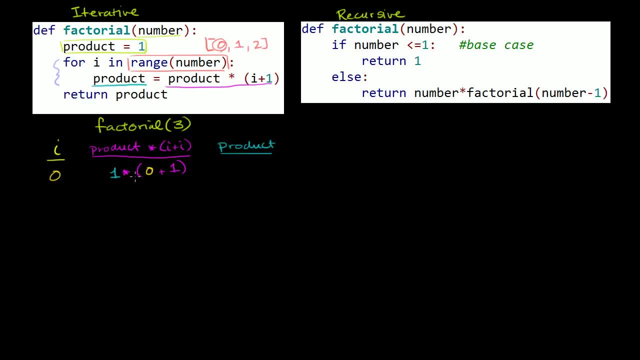 is essentially this evaluated. We have it right here: Product is equal to all of this business, And so our new value is 1.. So 1 times 0 plus 1, well, that's just 1 times 1.. And that's just going to be 1.. 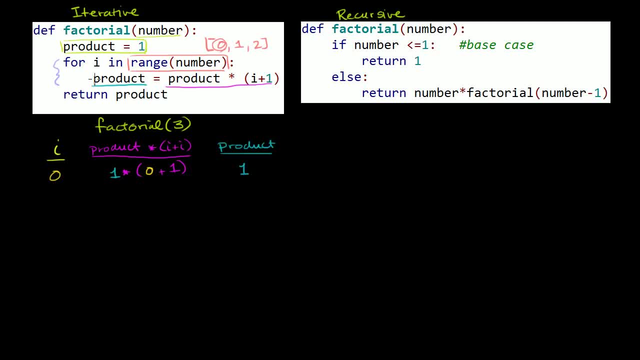 And that's all we had inside the for loop clause, because that's the only stuff that was indented within this for loop. And so then we go back up. So then we go back up and we're going to iterate through the next iteration of our loop. 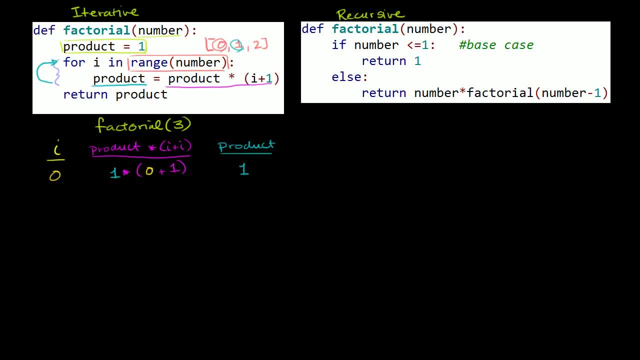 I guess you could say: And now i is going to be assigned to 1.. So now i is going to be 1. This expression over here we're going to take our old product. Product is still 1.. So product is 1.. 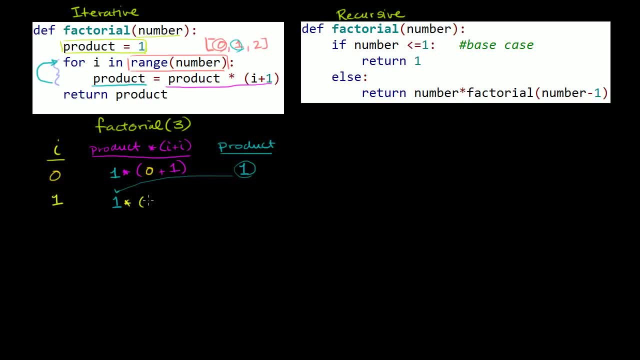 And it's going to be times i, which is now 1, plus 1.. And what's this going to be equal to? Well, if you evaluate all of this, you get 1 times 2.. So now the new value for product is 2,. 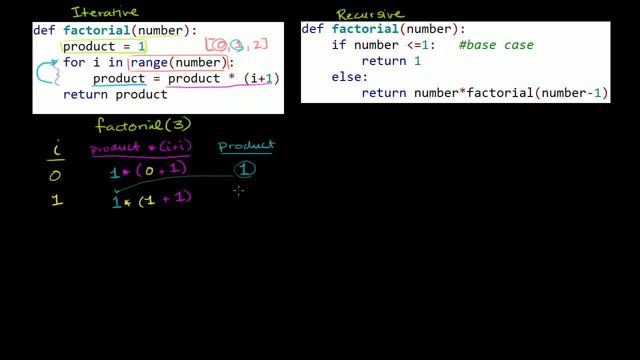 after our second iteration through the loop, our second pass through the loop. Now it will go back to the beginning of the for loop And i will be assigned to the next element in the list. It will now be assigned to 2.. So i is now 2.. 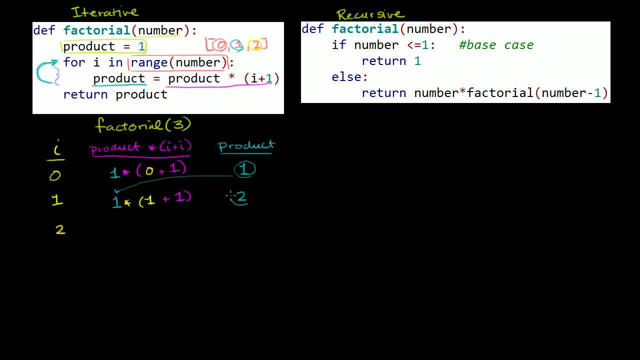 This thing over here. it's going to be product. Well, product is now 2.. So it's going to be 2 times i. Well, i is now 2, plus 1.. And so what does this see? This is 2 times 3, or 6.. 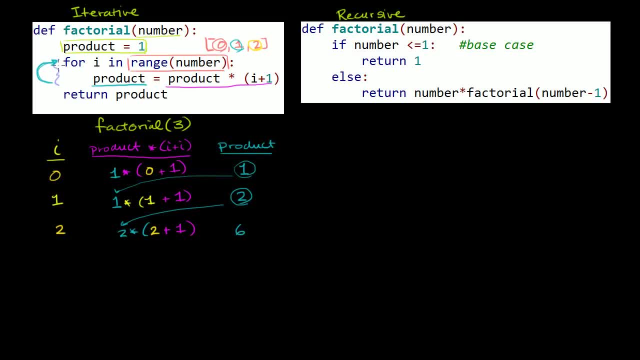 And then it will go and say: OK, can we assign i to any more elements in this? No, we've run out of elements. So now we break out of the for loop And we just return the product Or the variable product, what it's referring to. 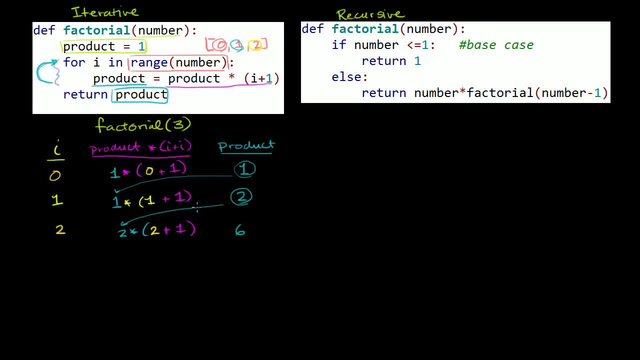 and that's what I should really say- where we should return the value that product is referring to, And that value is 6.. So when you call factorial 3, it will return 6.. So if you were to say factorial, if you say factorial, 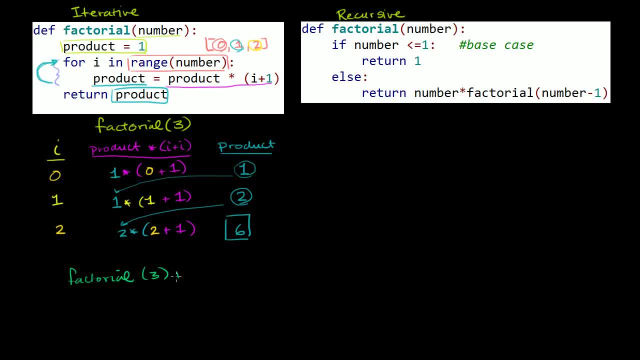 factorial of 3 plus factorial of 3, and you were to evaluate this expression, this expression would evaluate to 6.. And this expression over here would evaluate to 6, because that's what the function will return. And then you would add those up and they would evaluate to 12.. 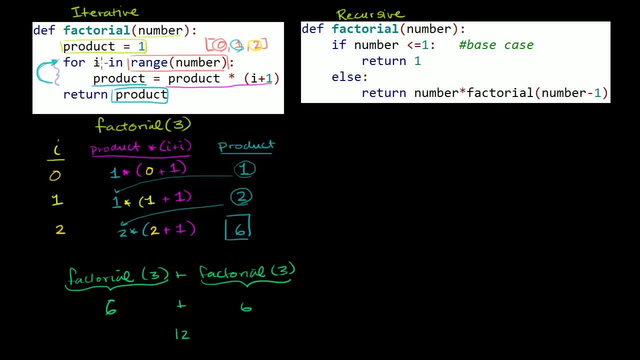 So this is why we call it iterative. We kept iterating through the same set of instructions. Now let's compare the recursive definition, And this is iterative. This one's a little bit more fun in a lot of ways. So once again, we're going to call factorial of 3.. 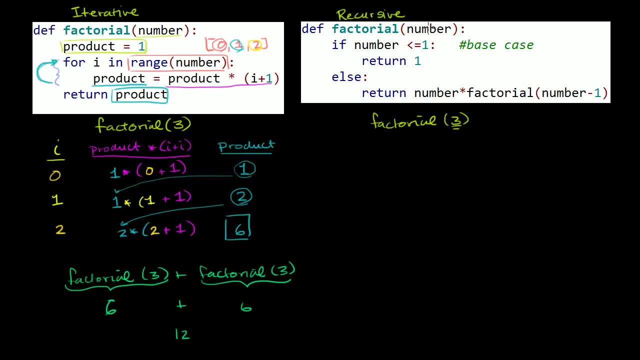 So 3 is our argument. That's the value that number will refer to. It'll take on, And it says if number is less than or equal to 1.. Well, 3 is not less than or equal to 1.. 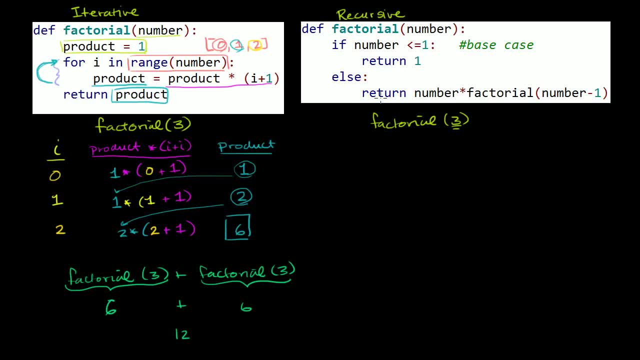 So we're not going to do this part over here. We're going to do the else clause. So we're going to return number, So we're going to want to return number times, factorial of all of this. So this is going to evaluate, to 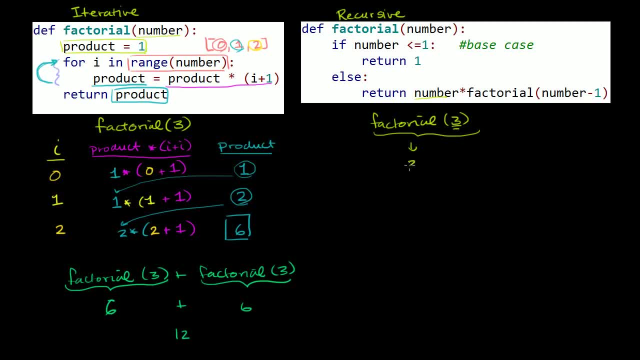 This is going to evaluate to Number which is 3.. That's the argument we passed Times factorial of number minus 1.. Well, number minus 1 is going to evaluate to 2.. 3 minus 1 is 2.. 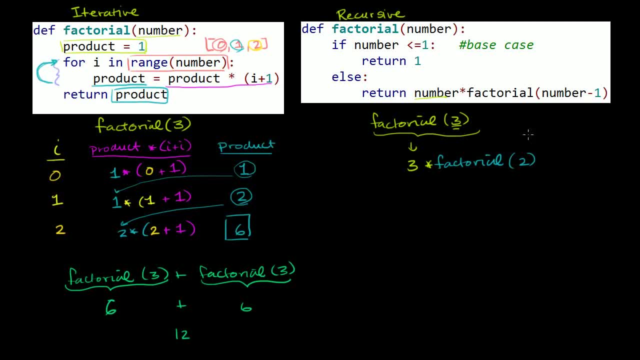 So times factorial of 2.. Well, that's just another function called a factorial. So we go back. OK, factorial, But now the argument is 2.. So number is 2. We go here. If number is less than or equal to 1, do this.